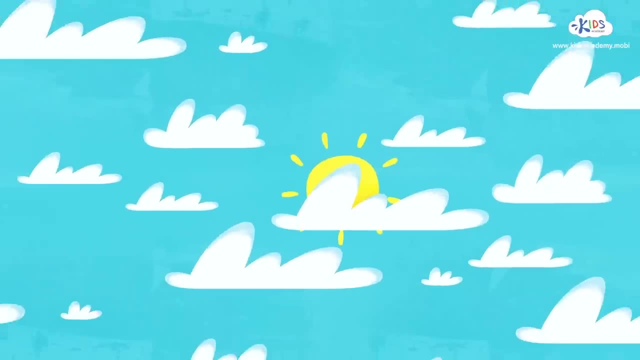 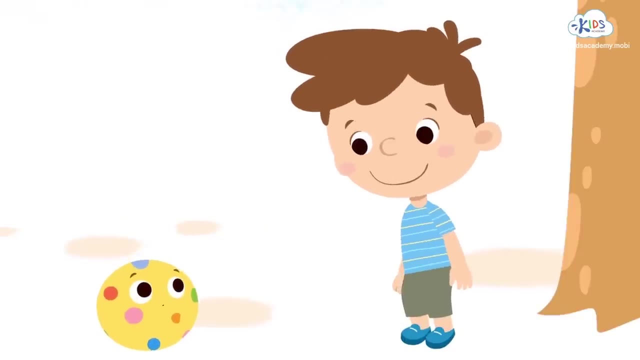 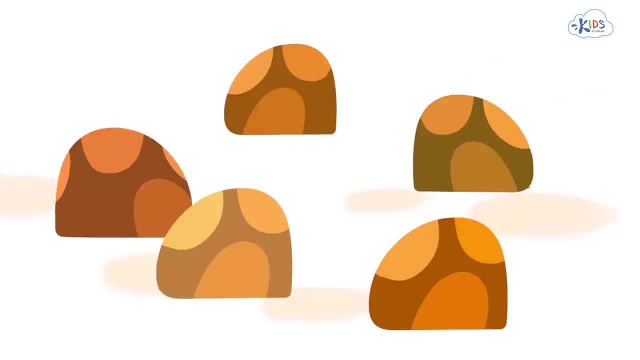 How many is lots? I don't know. The sky is so huge, It's hard to count them. And how many colorful dots do I have? It's hard to count them too. You jump very quickly. Well then, let's count these stones. They lie still. One, two, three. 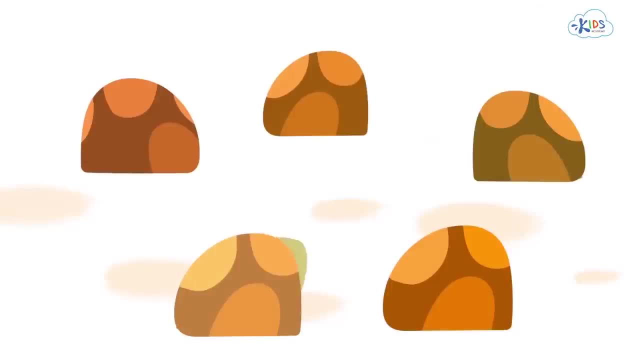 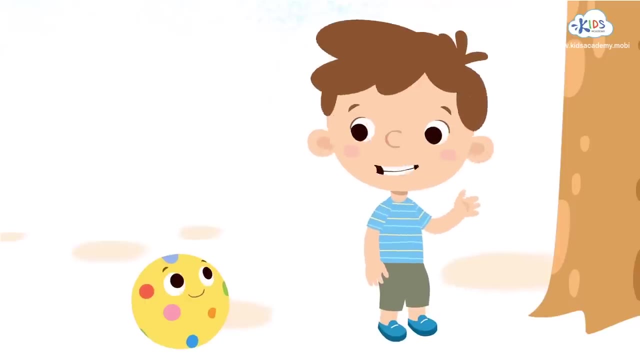 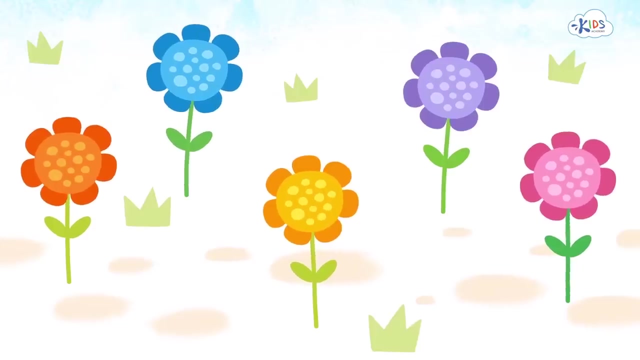 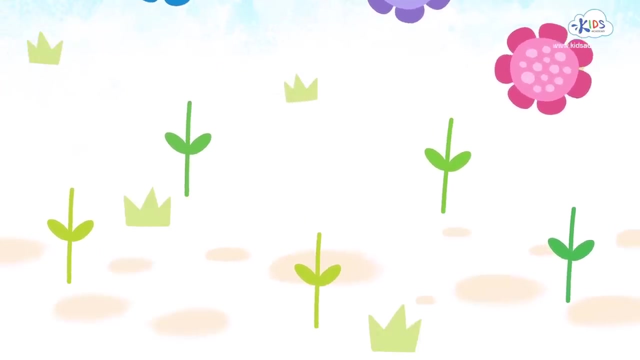 four, five, Wow, They are alive. It's turtles. They are hungry. Let's pick a flower for each of them. Turtles love to eat flowers. Hey, tell us, How many flowers do we need to treat the turtles? 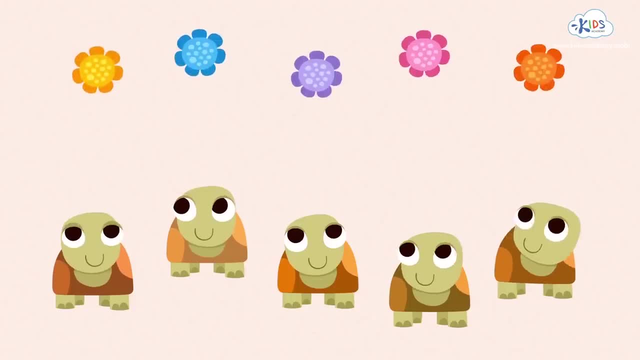 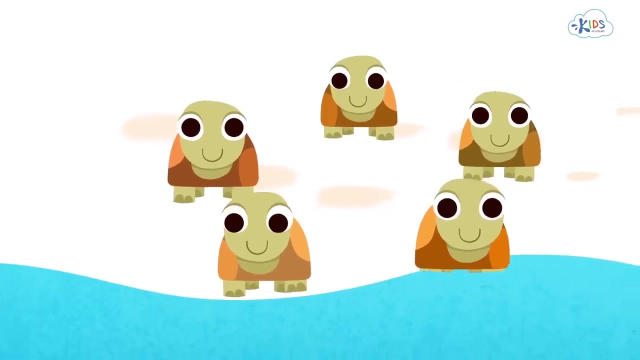 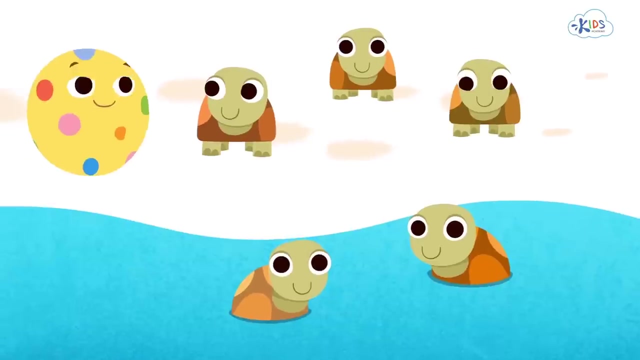 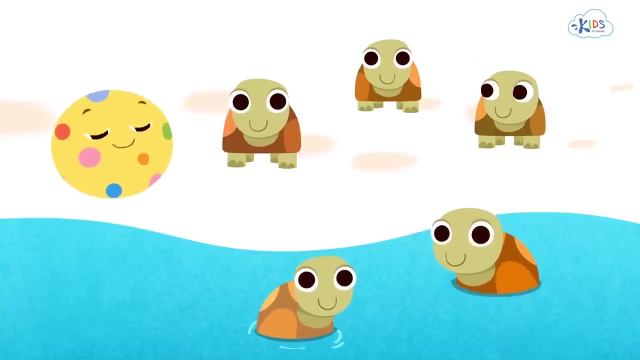 Five, Because there are five turtles: One, two, three, four, five. Bally solve a problem: How many turtles stay on the shore and how many swim in the water? One, two, three. One, two, Three turtles lie in the grass and two turtles are in the water. 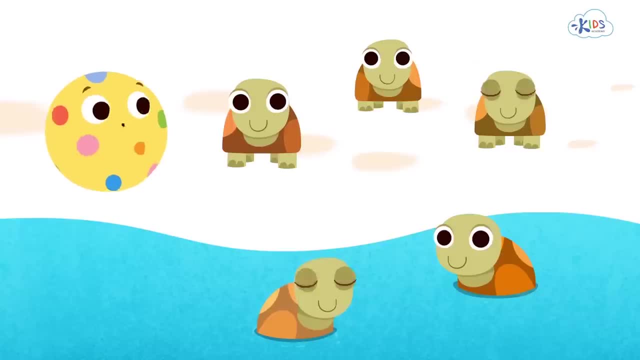 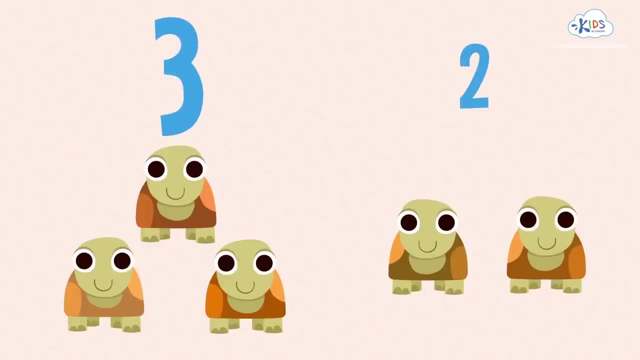 Which number is larger? There are more turtles in the grass, So I think number three is larger than number two. Number two is not the same. Number two is larger than number three. Number two is not the same. Number two is larger than number two. Number two is not the same. Number two is not the same. Number two is not the same. 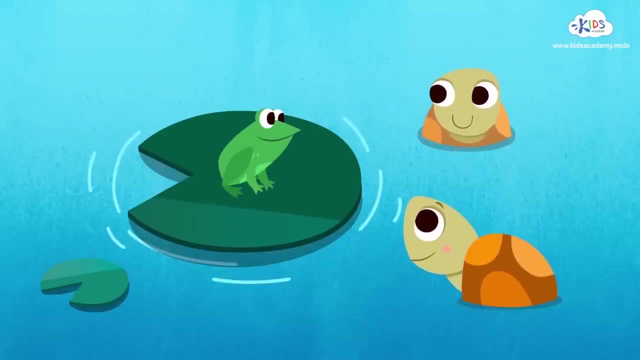 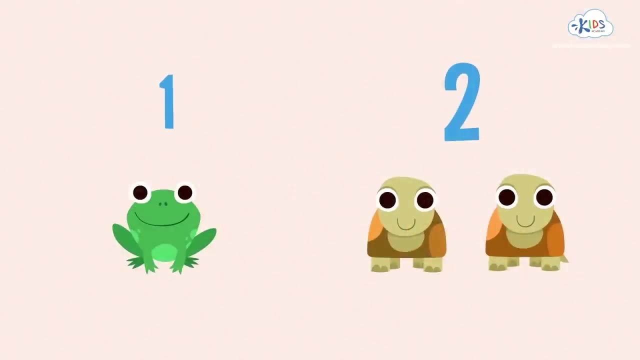 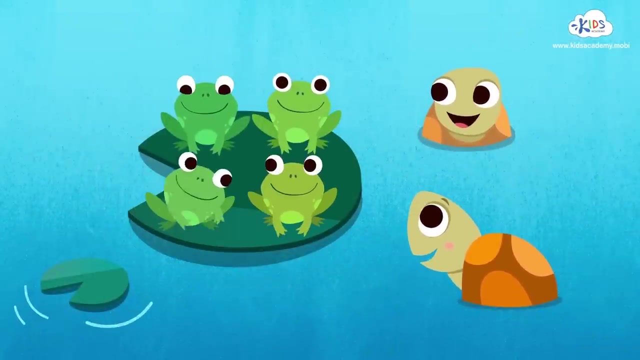 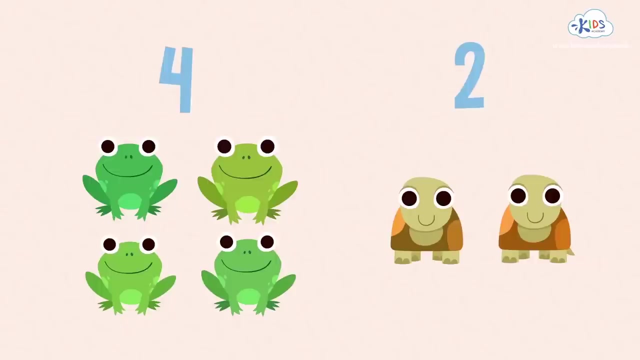